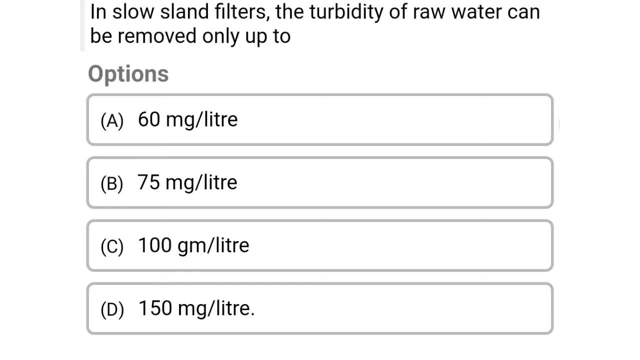 25 mg per litre, Option C: 100 mg per litre, Option D: 150 mg per litre. So the correct answer is Option A: 60 mg per litre. So next question: Biochemical oxygen demand BOD of safe drinking water must be Option A: nil, Option B: 5, Option C: 10. 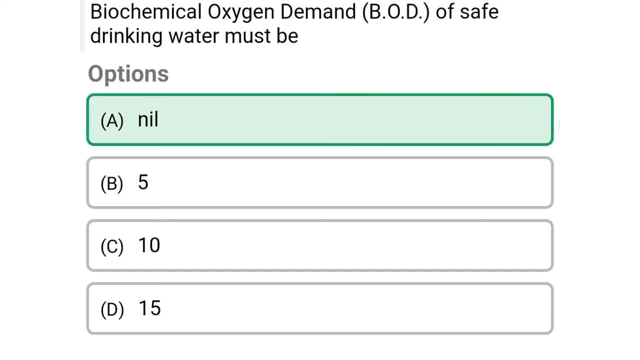 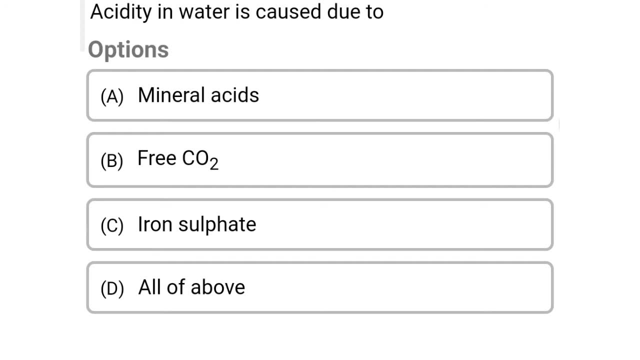 Option D 15. So the correct answer is Option A- nil. So next question: Acidity in water is caused due to Option A- mineral acids. Option B- free CO2. Option C- iron sulphate. Option D- aldehyde. So the correct answer is Option D, aldehyde. So next question: The transitional middle portion of logistic. 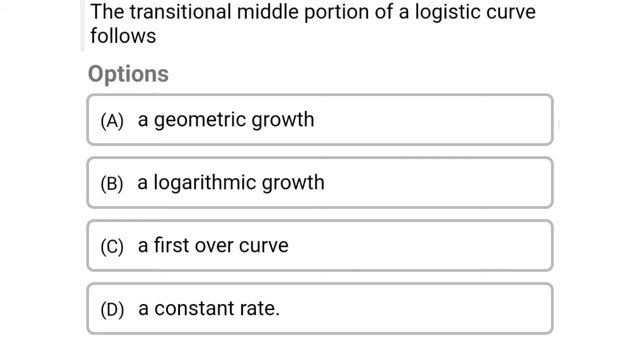 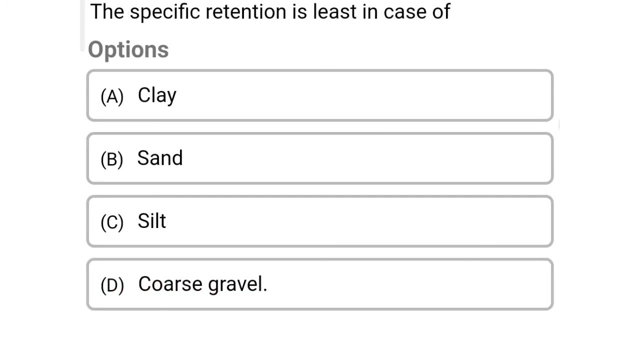 curve follows Option A a geometric growth. Option B a logarithmic growth. Option C a first over curve. Option D a constant rate. So the correct answer is Option D a constant rate. So next question: The specific retention is least in case of Option A clay, Option B sand. 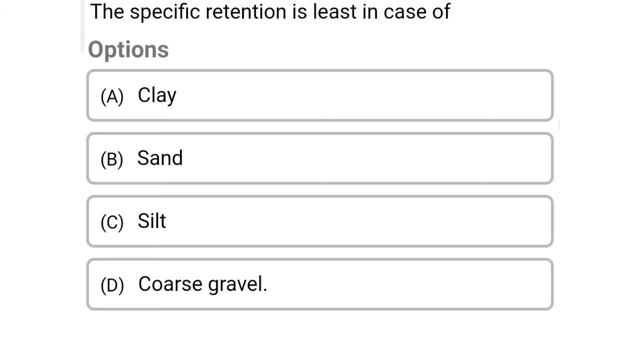 Option C- silt. Option D- coarse gravel. So the correct answer is Option D, coarse gravel. So next question: BOD of treated water should be Option A- 10 ppm. Option B- 25 ppm. Option C- 20 ppm. Option D- nil. So the correct answer is Option D, nil. 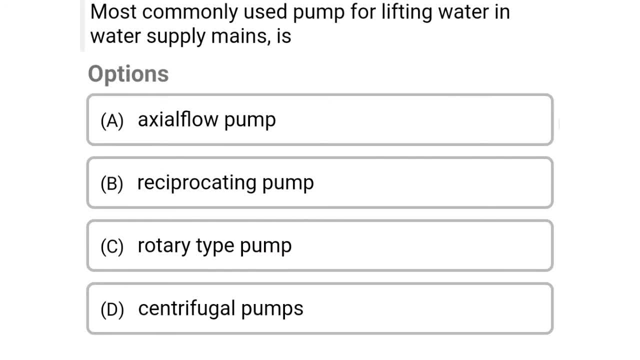 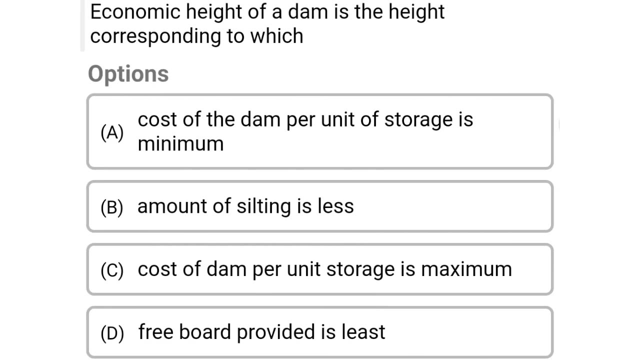 So next question: Most commonly used pump for lifting water in water supply mains is Option A- axial flow pump, Option B- reciprocating pump. Option C- rotary type Pump. Option D- centrifugal pump. So the correct answer is Option A, axial flow pump. So next question: Economic height of the dam is height corresponding. 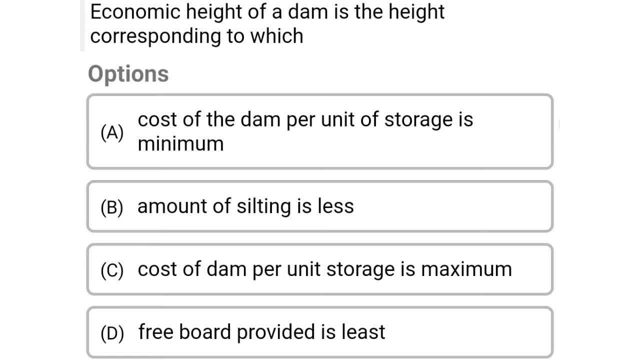 to which? Option A- cost of the dam per unit of storage is minimum. Option B: amount of silting is less. Option C- cost of dam per unit storage is maximum. Option D- free board provider. it is least. so the correct answer is option a- cost of the dam per. 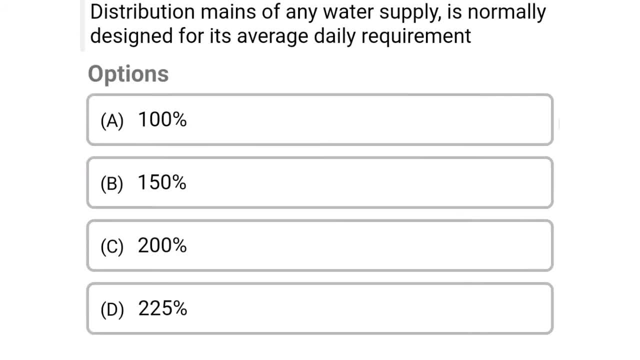 unit of storage is minimum. so next question: distribution mains of any water supply is normally designed for its average daily requirement: option a: 100. option B: 150 percentage. option C 200 percentage. option D: 225 percentage. so the correct answer is option D, 225 percentage. so next question: a high. 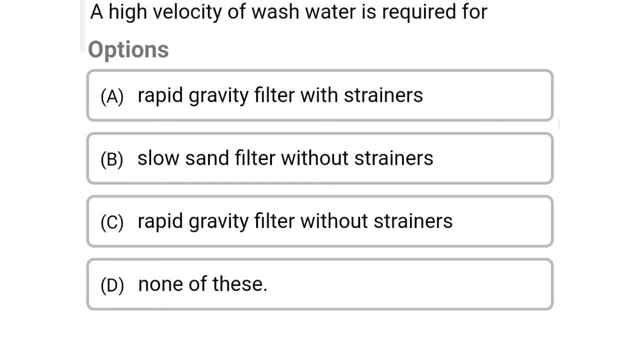 velocity of wash water is required for option a- rapid gravity filter with strainers. option B- slow sand filters without strainers. option C- rapid gravity filter without strainers. option D- none of this. so the correct answer is option B- slow sand filter without strainers. so next question: in distribution pipes: 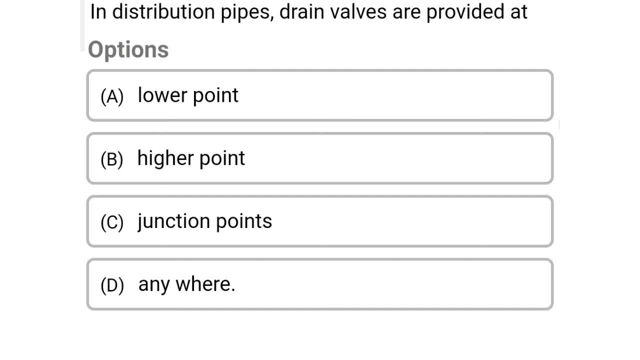 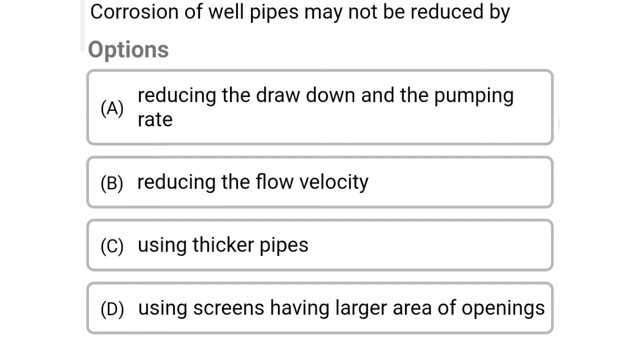 drain walls are provided at option a- lower point, option B- higher point, option C, junction points, option D- anywhere. so the correct answer answer is option a, lower point. so next question: corrosion of weld pipes may not be reduced by option a, reducing the drawdown and the pumping rate, option b- reducing the flow velocity, option. 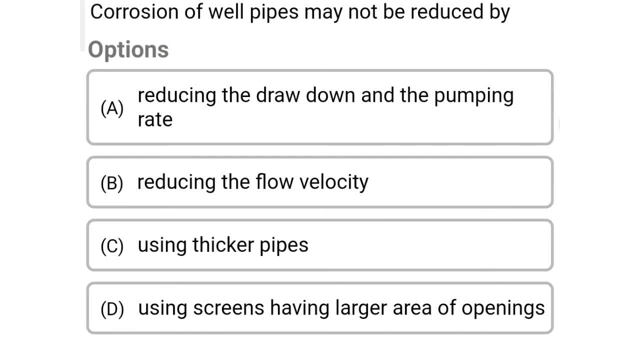 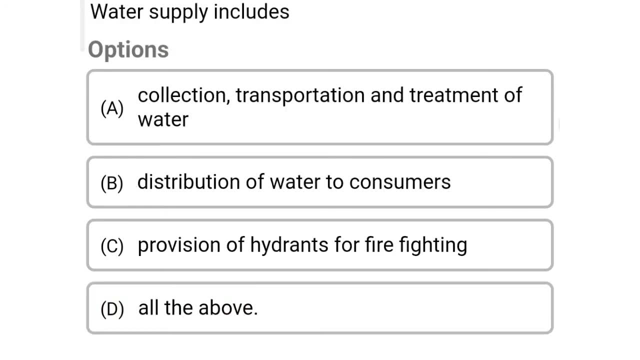 c- using thicker pipes. option d- using screens having large area of openings. so the correct answer is option d- using screens having large area of openings. so next question: water supply includes: option a- collection, transportation and treatment of water. option d- sorry. option b- distribution of water to consumers. option c- provision of hydrants for firefighting option. 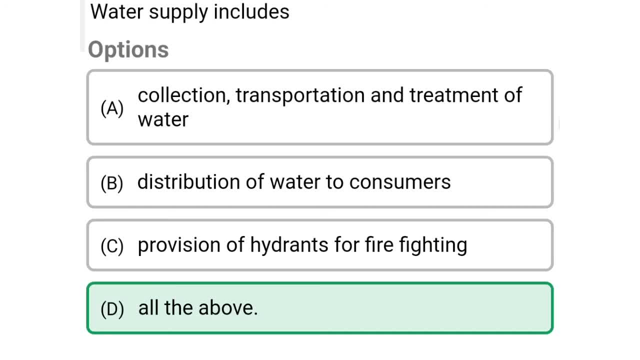 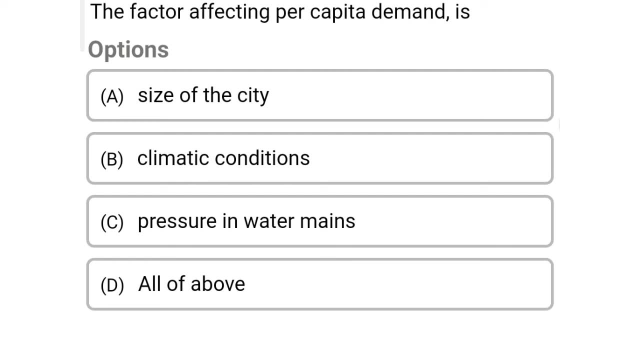 d- all they book. so the correct answer is option d- all they book. so next question: the factor affecting per capita demand is option a- size of the city. option b- climatic condition. option c- pressure in water mains. option d- all they book. so the correct answer is option d. 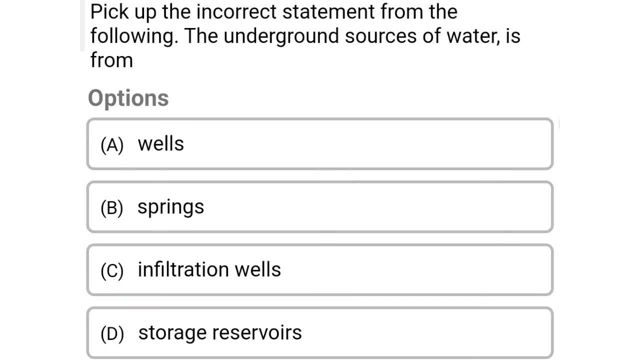 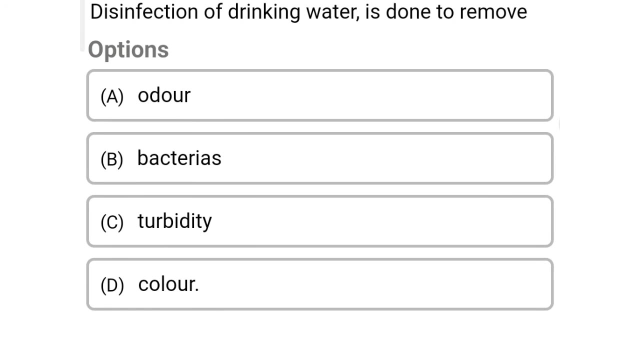 all they book. so next question: pick up the incorrect statement from the following: the underground sources of water is option a- wells. option b- springs. option c- infiltration wells. option d- storage reservoirs. so the correct answer is option d, storage reservoir. so next question: disinfection of drinking water is done to remove- option a- order. option b- bacterias. option c. 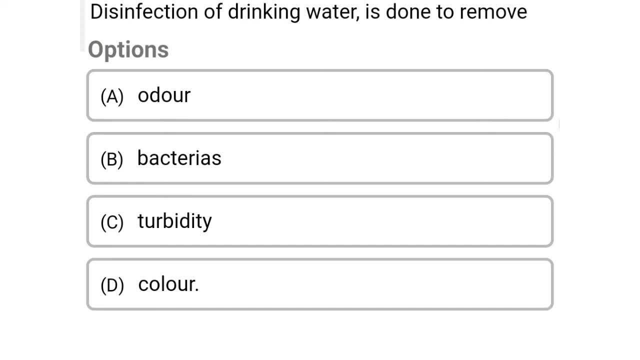 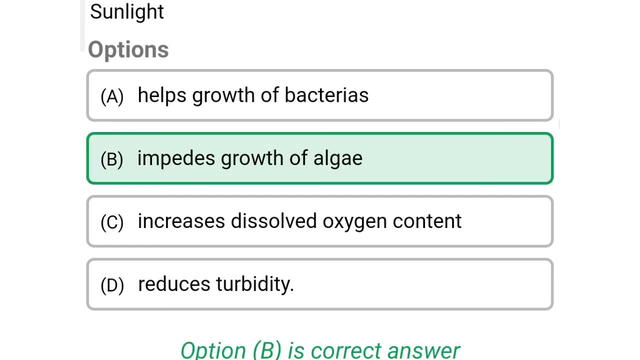 turbidity. option d- color. so the correct answer is option b- bacterias. so next question: sunlight- option a- help growth of bacterias. option b: impairs growth of algaes. option c: increased dissolved oxygen content. option d: reduced turbidity. so the correct answer is option b. 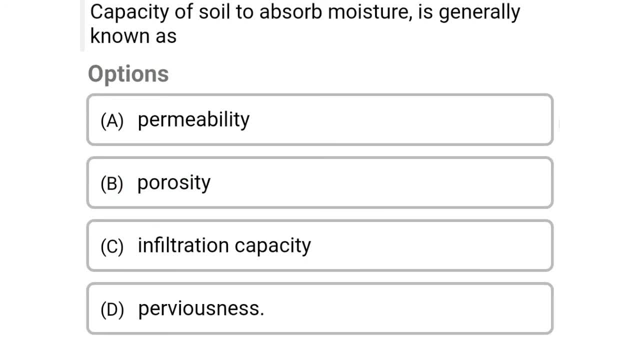 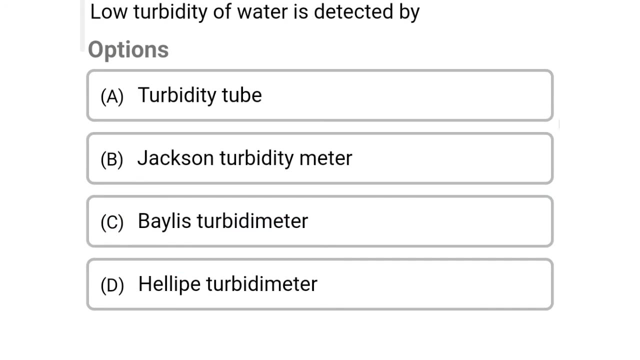 impairs growth of algaes. so next question: capacity of soil to absorb moisture is generally known as option a- permeability, option b- porosity, option c- infiltration capacity, option d- perviousness. so the correct answer is option c, infiltration capacity. next question: low turbidity of water is detected by option a, turbidity tube, option b- jackson. 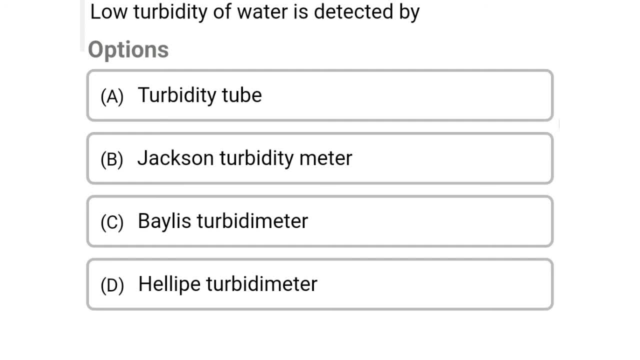 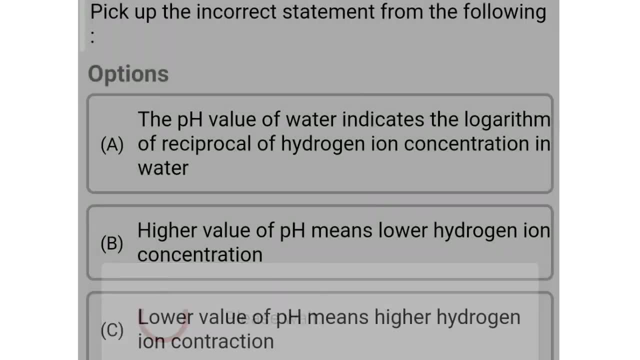 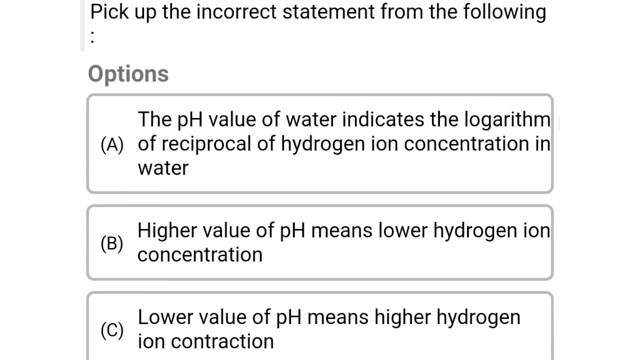 turbidity meter. option c- bayless turbidity meter. option d- helip turbidity meter. so the correct answer is option c- bayless turbidity meter. so next question, pick up the incorrect statement from the following. option a: the ph value of water indicates the logarithm of reciprocal of. 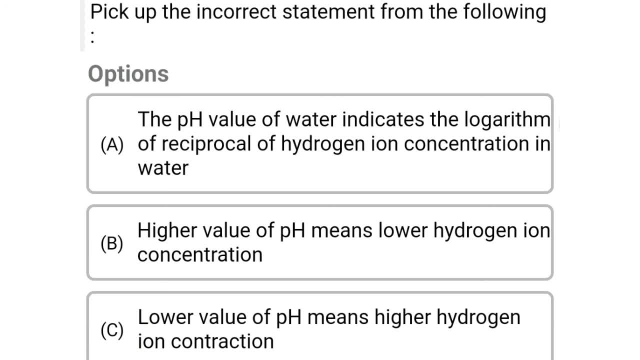 hydrogen ions concentration in water. option b: higher value of ph means lower hydrogen ion. in opposition c: lower value of ph means higher hydrogen ion concentration ups and the lower value of ph gives alkaline solution. so the correct answer is option d: lower value of ph gives alkaline. 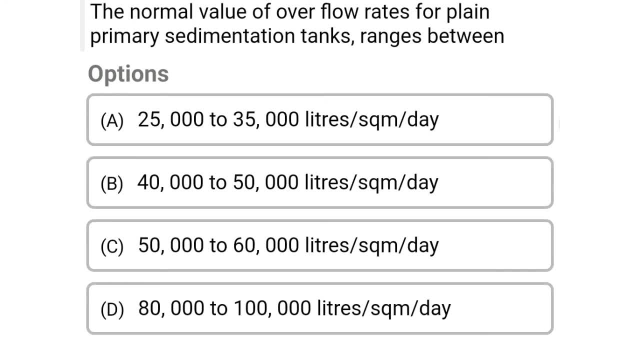 solution. so next question: the normal value of overflow rates for blind primary sedimentation tanks ranges between: option e: 25 000 to 35 000 liter per square meter per day. option b: 40 000 to 50 000ivotable per reconibated per meter per day on different sources. order dark: an biogas tank min. 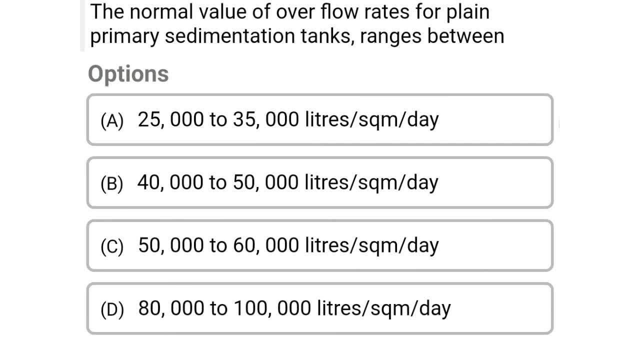 C: 50,000 to 60,000 liters per square meter per day. Option D: 80,000 to 100,000 liters per square meter per day. So the correct answer is Option B: 40,000 to 50,000 liters per square. 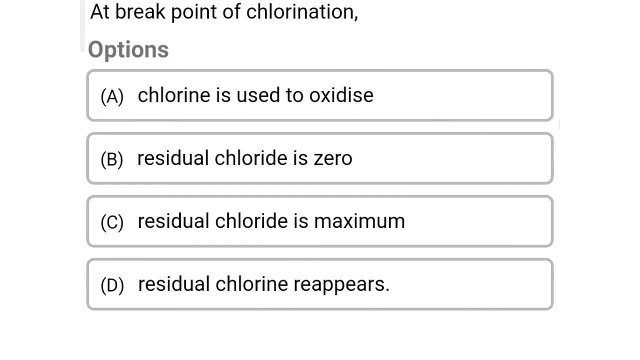 meter per day. So next question, At breakpoint of chlorination. Option A- Chlorine is used to oxidize. Option B- Residual chloride is zero. Option C: Residual chloride is maximum. Option D: Residual chlorine reappears. So the correct answer is Option D- Residual chlorine reappears. 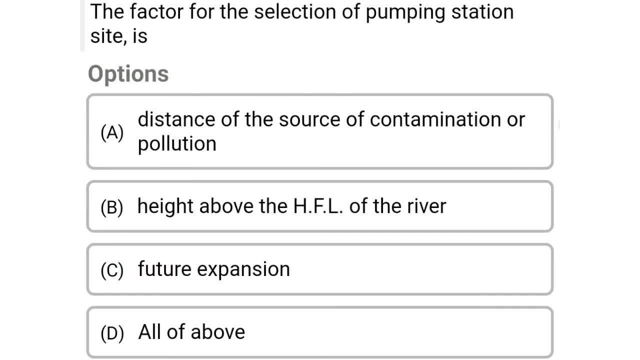 So next question, The factor for the selection of pumping station at site is: Option A: Distance of the source of contamination or pollution. Option B: Height of above HFL of the river. Option C: Future expansion. Option D: All the above. So the correct answer is Option D, All the above. Again. we will see in next video, Thank you,